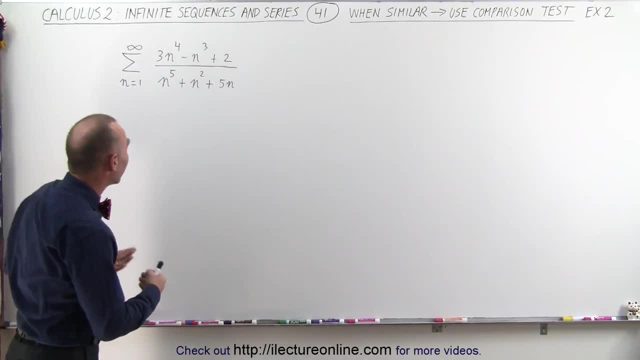 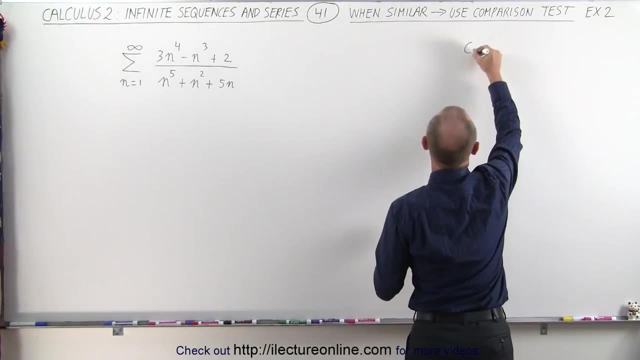 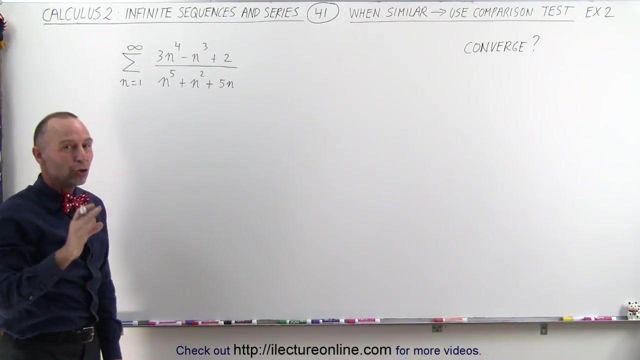 Welcome to Electron Line. Sometimes you're faced with an infinite sum like this and you wonder: how do you tell that it converges or diverges? So that's the question: Does it converge or does it diverge? Well, what you can say is that it looks very similar to something like this. So it is. 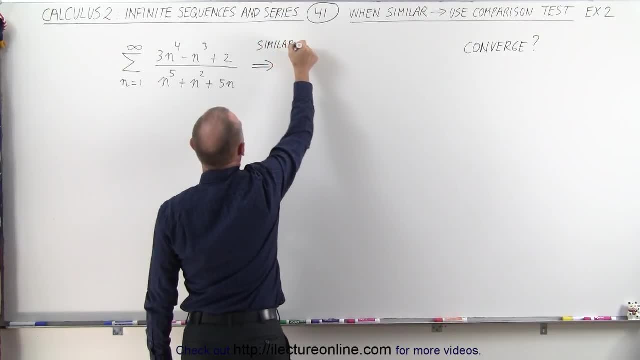 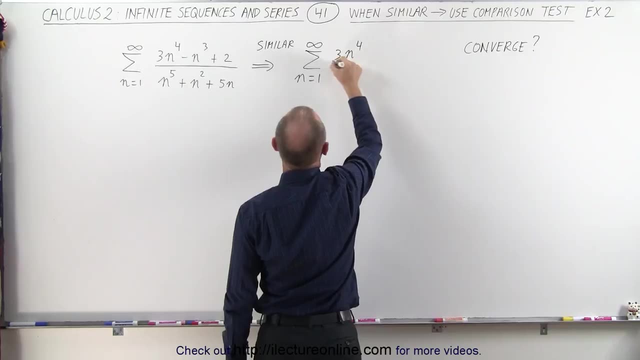 similar to the following: An infinite sum from n equals 1 to infinity, of 3n to the 4th, divided by n to the 5th, And we drop off the other two terms in the numerator and the other two terms in the. 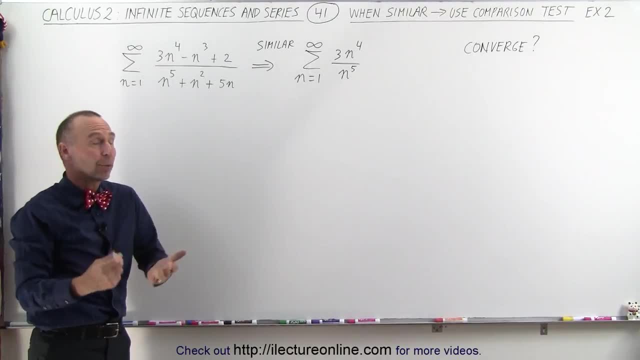 denominator. You may say: well, why do I do that, Aren't they important? Well, it turns out, as n becomes large, and it will become large quickly, n to the fifth and n to the fourth will far over power, the value of the numerator. So this is the cost of the last sum. The cost of the last sum is: 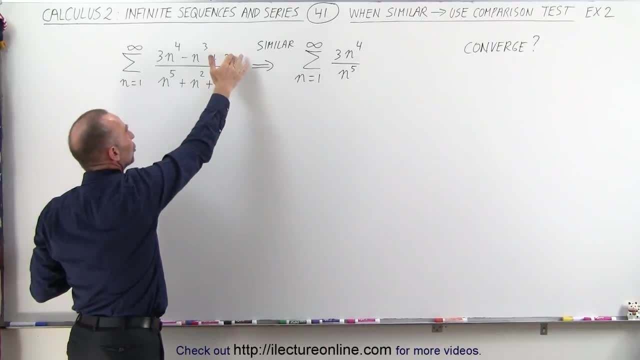 the total value of the numerator and denominator. You're going to ask yourself: well, why do I do that? that n to the third and n to the second will get, and especially 2 and 5 to the n, So they become insignificant very quickly. so only this drives the infinite series as n becomes large and so 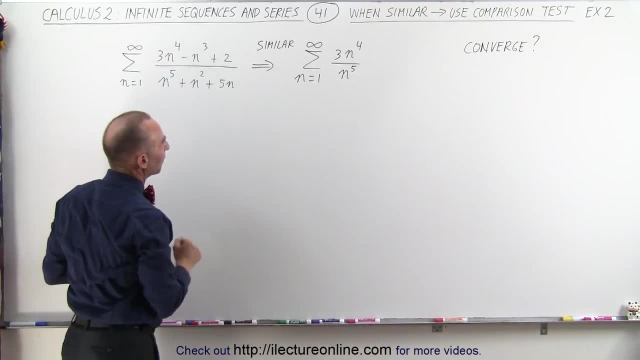 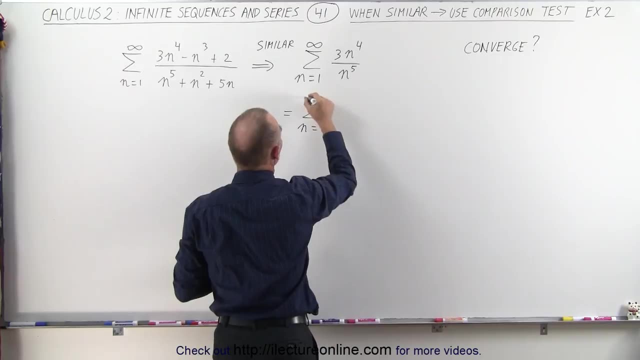 therefore, this will determine whether or not it converges or not. So when we look at this, we can say: well, this is equal to the infinite sum from n equals 1, to infinity of 3 times n, to the 4 divided by n, to the fifth, which is 1 over n, and now we have an infinite series of 3 times. 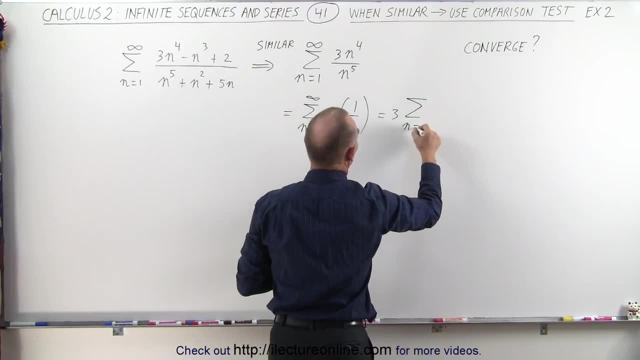 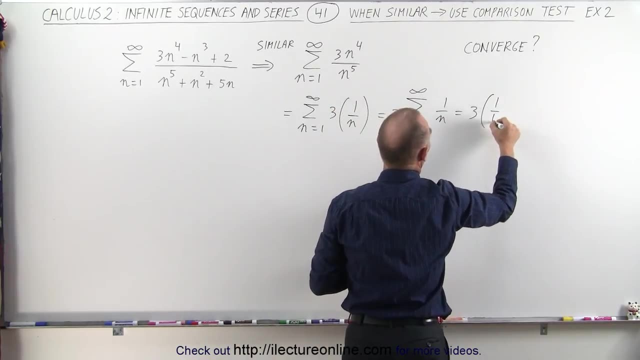 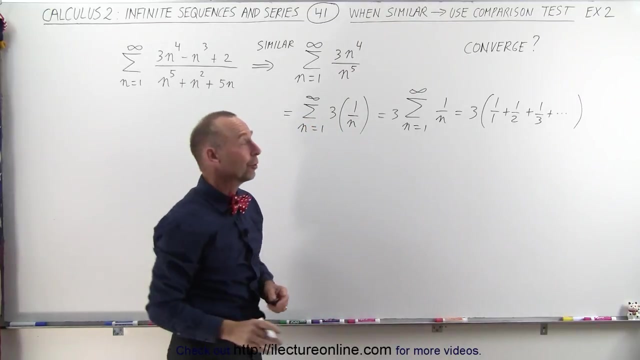 the sum from n equals 1 to infinity, of 1 over n, which is equal to 3 times 1 over 1 plus 1 over 2 plus 1 over 3 plus, and so forth. and we know that that series does not converge. so if that doesn't, 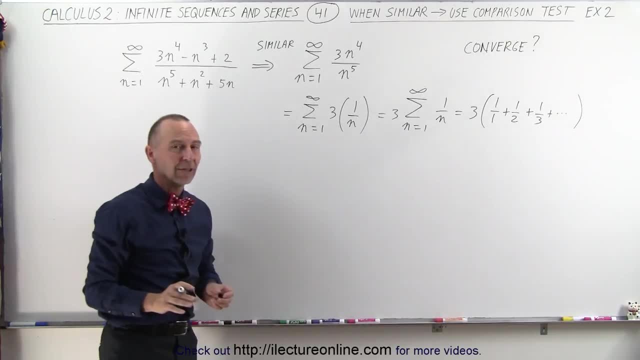 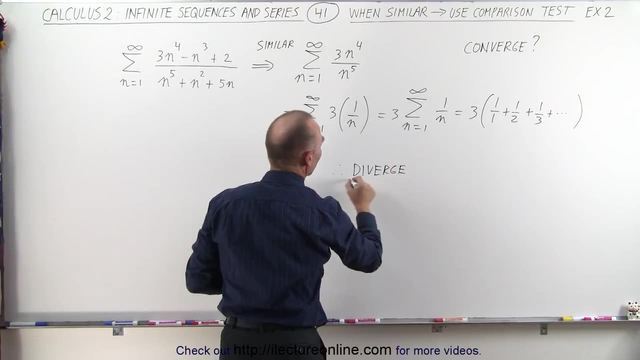 converge and in those small terms at the end will not make any difference. it will not converge. So we have an infinite series of 3 times the sum from n equals 1 to infinity of 1 over n. so therefore we can say that this series will diverge and again using the comparison test, 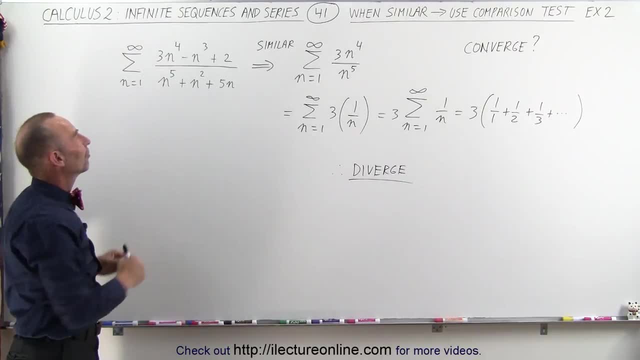 is often a very good way, keeping from trying to do something very difficult and turning it into something that's rather simple, and that's how it's done.